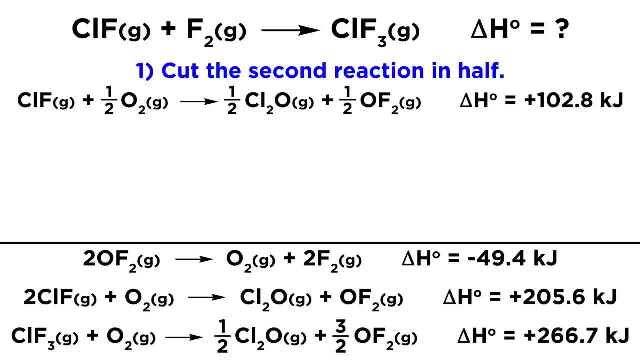 becomes one half O2.. Cl2O becomes one half Cl2O And OF2 becomes one half OF2.. Now we mustn't forget to cut that delta H in half as well, because we're cutting all the stoichiometric coefficients in half, That means the delta H will be half as much as well. So 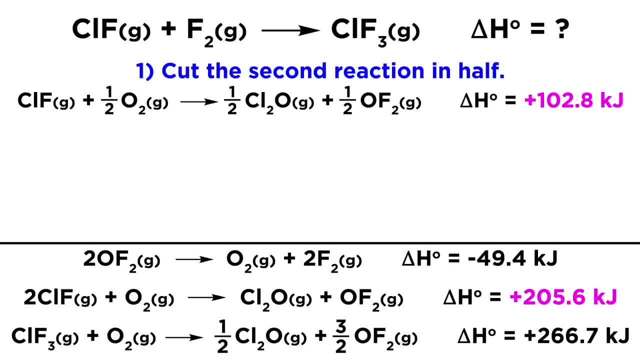 205.6 becomes 102.8.. Now what's next? We need F2.. We need F2 as a reactant. So where's F2?? Well, over here we have two F2, and we have it as a product, And that's the only place F2 is. So we 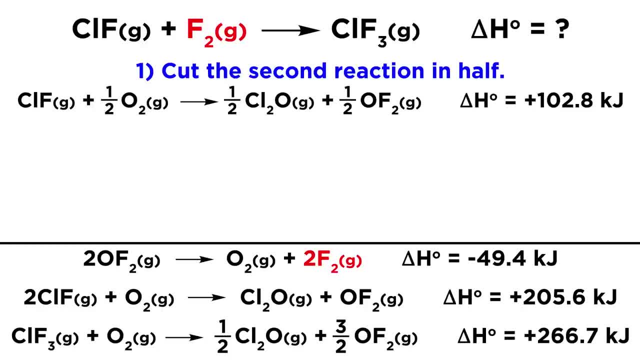 know we need to use this equation. So what are we going to do? We need F2 as a reactant, but here we have two F2 as a product. So what we need to do is we need to take this first reaction. We have to. 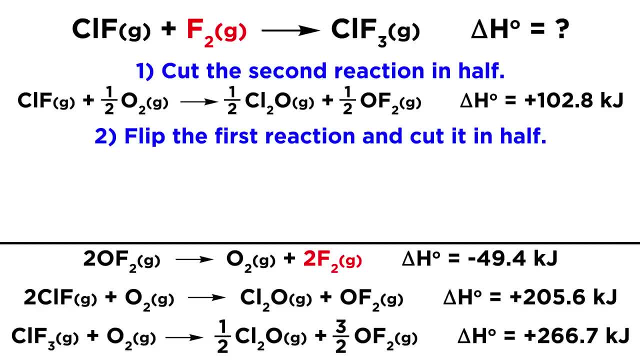 flip it so that the products become reactants and the reactants become the products. And we also have to cut it in half. So we have to do two manipulations here. So let's do that Products become the reactants, So O2 as a product becomes one half O2 as a reactant. 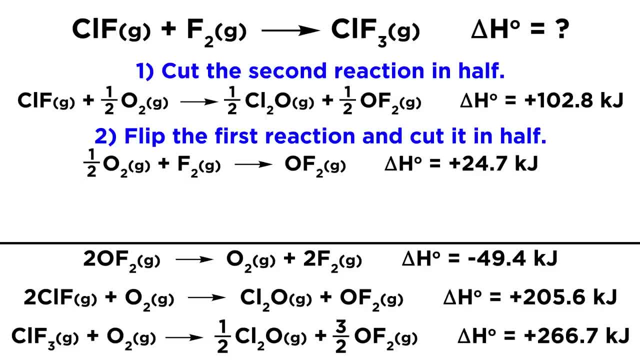 And then two F2 as a product becomes F2 as a reactant, And then two OF2 as a reactant becomes one OF2 as a product. So we have flipped it and we have cut it in half. And don't forget, we have to also manipulate the delta H value in the corresponding way. 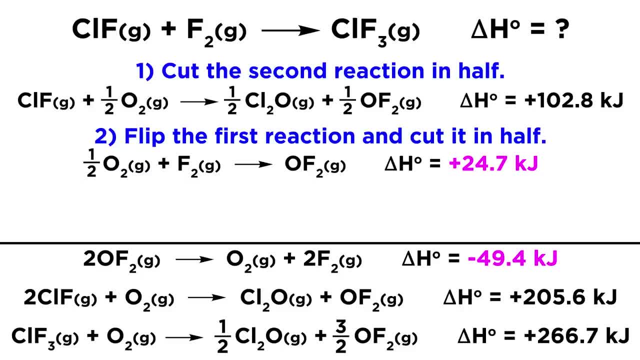 So when we flip it, whenever we make the products the reactants and the reactants the products, all we have to do is flip the sign. So we took our negative 49.4 and we made it positive 49.4, but we also cut everything. 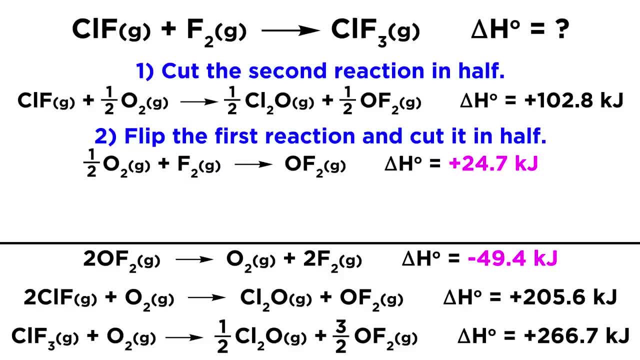 in half. So from positive 49.4, we went down to positive 24.7.. So that is the delta H value for this reaction. And lastly, we need ClF3 and we need it as a product. So where can we find it here? 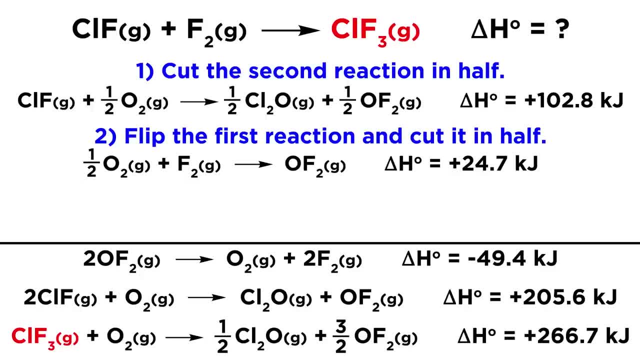 Well, this third reaction has ClF3, but it has it as a reactant. So what can we do? All we have to do is flip the third reaction. So let's do that now. So one half Cl2O as a product becomes a reactant. 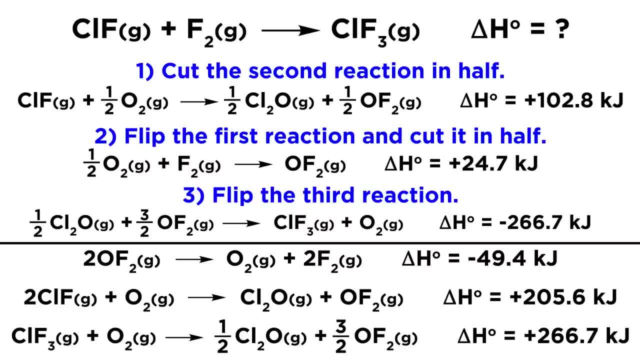 Three halves Of2 becomes a reactant, And then ClF3,, which was a reactant, is now a product, And O2 is also now a product. And once again, we can't forget- we have to take our delta H value. 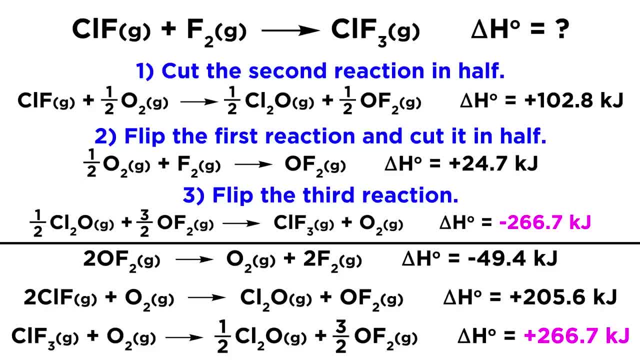 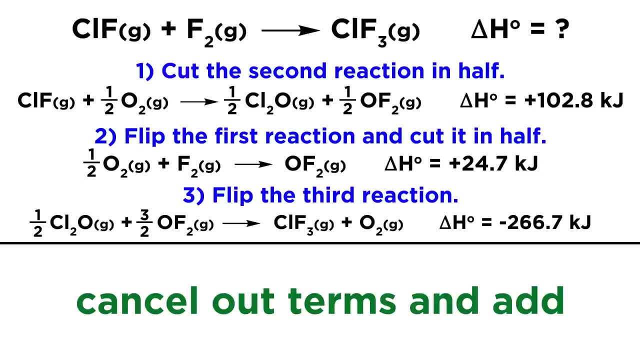 It was positive 266.7 because we flipped it. It is now negative 266.7 kilojoules, So we've got everything we need. So let's just check and make sure what cancels out. Let's make sure everything that we don't want in there is going to cancel out. 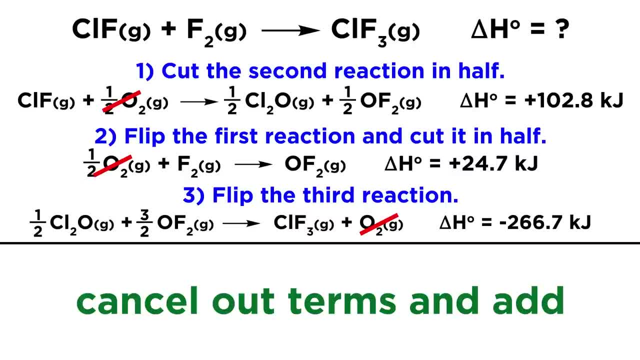 So what do we have? Well, on the left we have our delta H value. We have a half O2 in the first reaction, We have a half O2 in the second reaction. Those are both reactants. And then we have one O2 as a product in the third reaction. 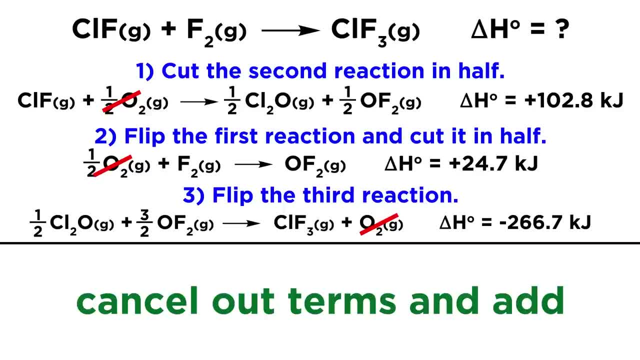 So half and half makes one, And then we have one on the right, So O2s all cancel out. Then we have one half Cl2O as a product in the first reaction And we have one half Cl2O as a reactant in the third reaction. 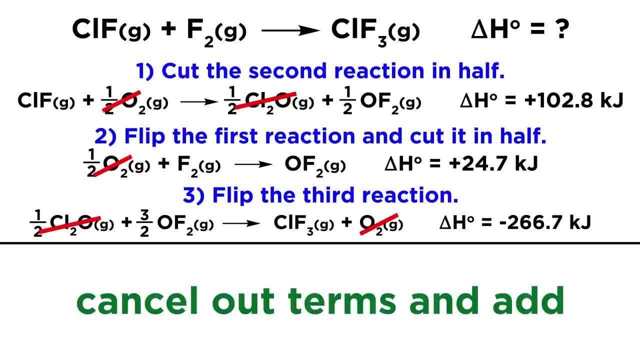 So those will also cancel out nicely. Then on the right we have one half OF2 in the first reaction, We have one OF2 in the second reaction And then in the third reaction we have three halves OF2 as a reactant. 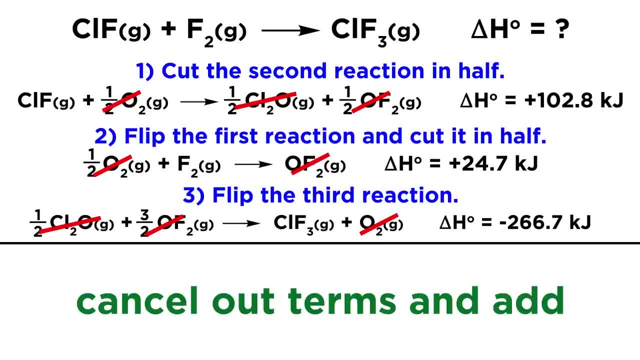 So three halves OF2 total as products and three halves as reactants, And so those will also cancel nicely. And what are we left with? We are left with just what we wanted. We've got ClF, We've got F2.. 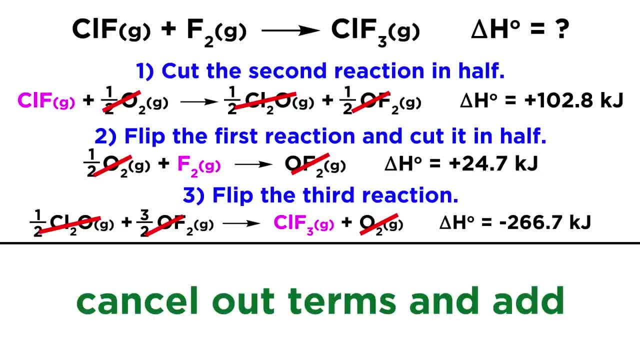 And we've got ClF3.. So that is what we wanted. We do end up with the reaction as listed at the top, So all we have to do is now add up the corresponding enthalpy data, And so for the first one, we've got 102.8. 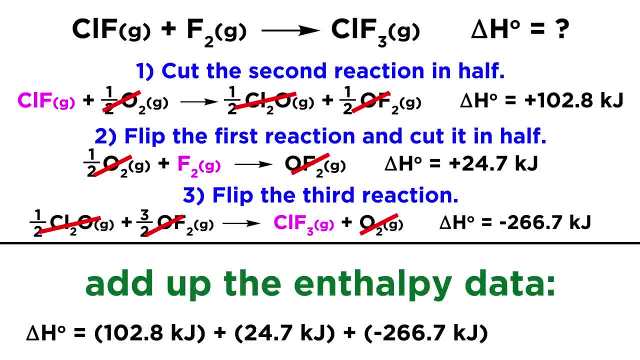 For the second one we've got 24.7.. And for the third one we've got negative 266.7.. So we put those in the calculator, add them up and we end up with negative 139.2 kilojoules. 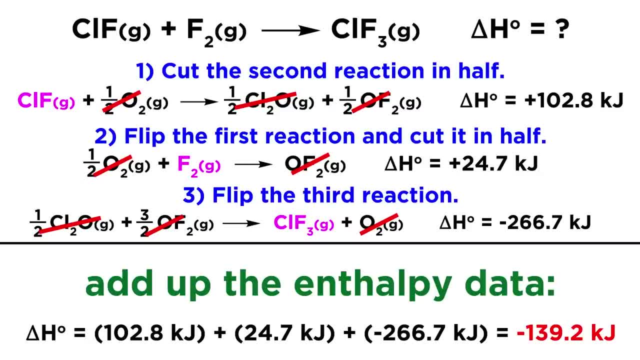 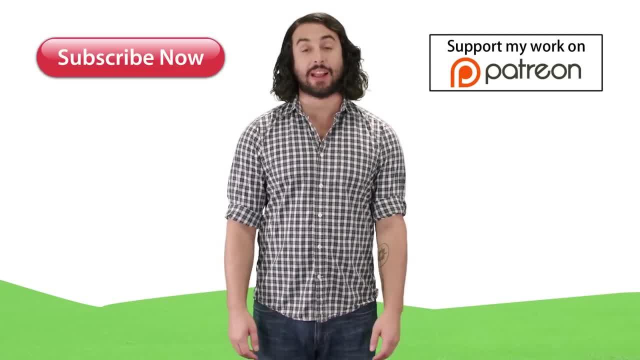 That will be the delta H for the reaction in question. Thanks for watching, guys. Subscribe to my channel for more tutorials, support me on patreon so I can keep making content and, as always, feel free to email me professordaveexplains at gmailcom.